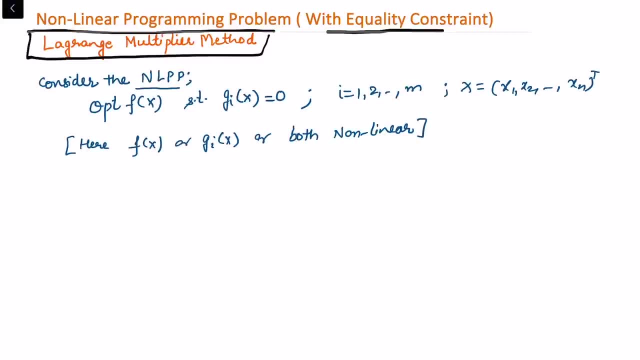 we consider nonlinear programming problem or simply nonlinear problem, where we have objective function without any constraint. So for optimizing nonlinear objective function without constraint, we have found the stationary point. and for finding the stationary point, So let's say, if I have a function f of x, this I want to optimize. So for 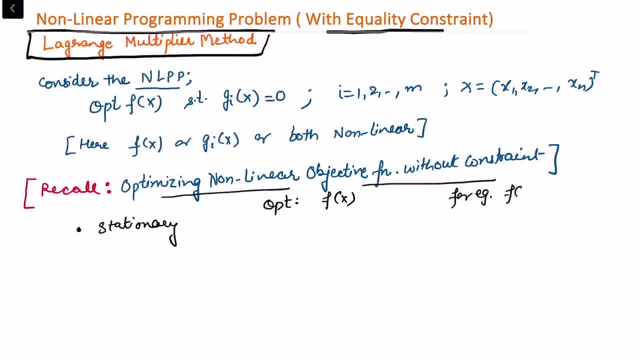 example, we may consider, say f of x is equal to x1 square plus 2x2 square, and then we can take, let's say, minus 2x2.. So there also we define fx into 2.. And then for Nonquadratic Data Forms, either this can be a quadratic form or this can be a nonquadratic form. 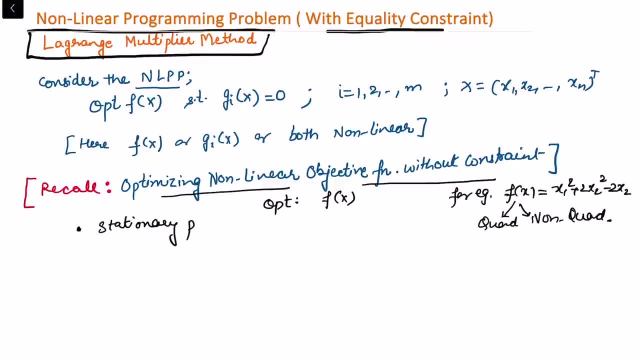 So, depending upon which this form is, we can then make the further steps. So we found the stationary point, which is curly F of with respect to curly xi equal to 0, and putting these all so in this question there are two variable: x1, x2.. So we will have curly f of with respect to curly x1 should be equal to zero and curly f of respect to 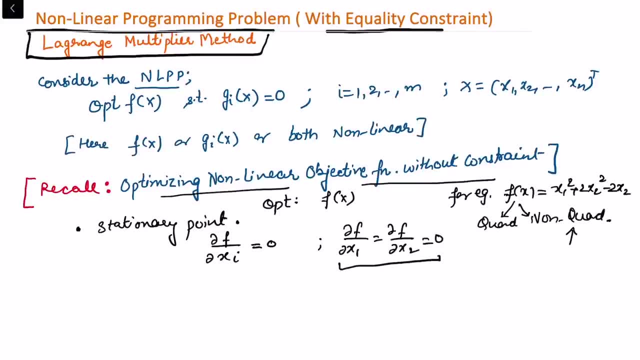 curly x2 should be zero. Solving these partial derivatives or these equations, we will find a stationary point which satisfied. now, this stationary point can be a point of maxima or minima, depending upon how the associated matrix is classified. so we did this point in the 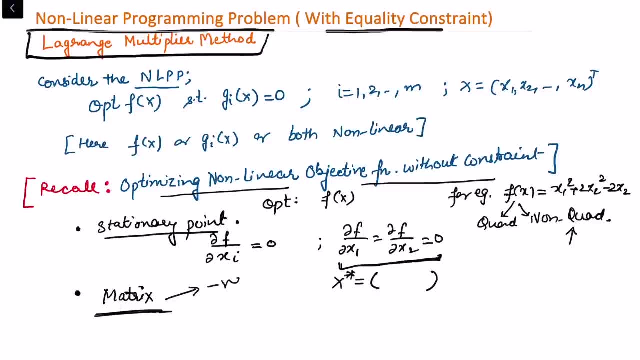 last video classification of the matrix point. if it is negative definite or if it is positive, definite will classify this into maximization or minimization. so the function will take the optimal value at this stationary point, depending upon what is the classification now. similar approach we will apply for the. 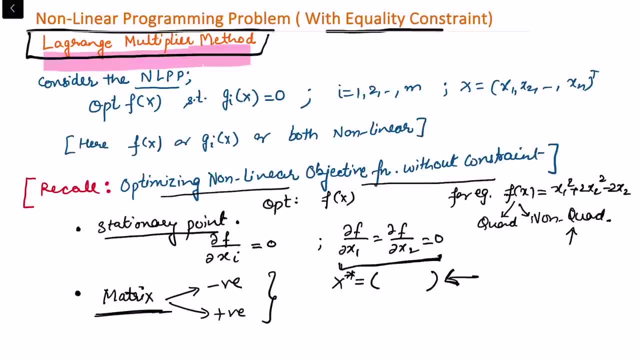 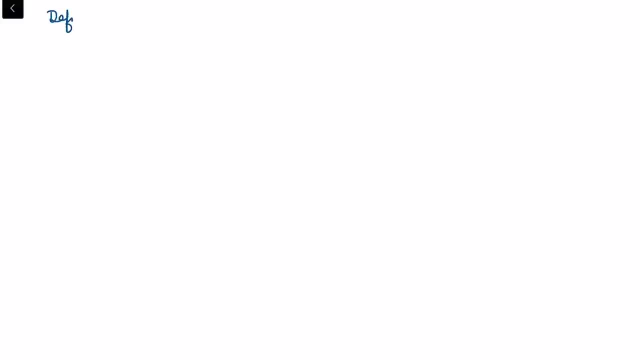 Lagrange multiplier method. but here we notice that we have a function separately and the constraints are separate. so using these two we will construct a Lagrange function, which would be a single function. so and then we will try to optimize that single function. so we now defined the Lagrange function. so 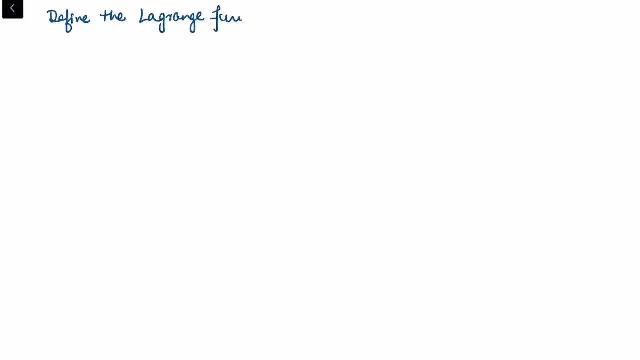 we'll call it as a Lagrange function and I denote this Lagrange function by L, capital X lambda. so capital X is a set of the small decision variables, small x as capital L, which is equal to x comma lambda. this is f of x, the original. 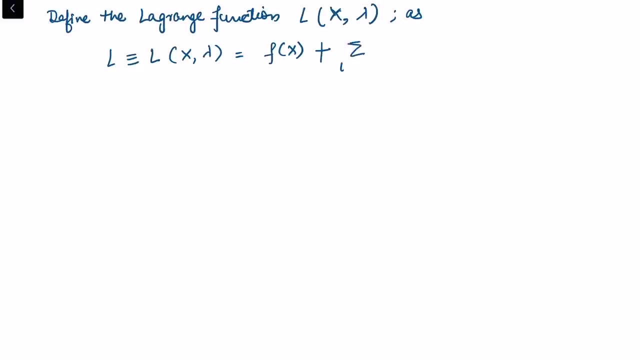 function plus summation i, varying from 1 to m, lambda i, g, i, x, and these lambda i's where these lambda I, these are called Lagrange multiplier. so from this objective functions and from the constraint have constructed a single objective function, and now we will apply our previous method. so here let me to take first an 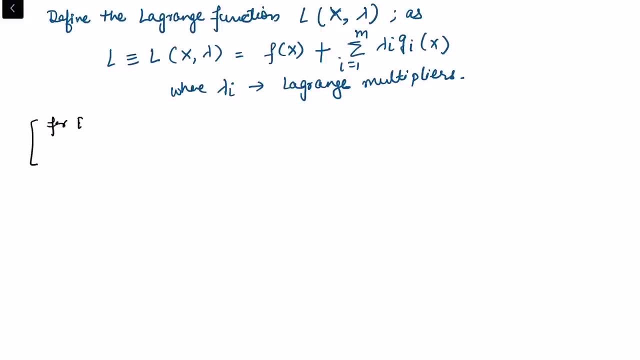 example how we constructed the Lagrange function. so, for example, we have an objective function that I want to optimize. so we can take optimum F of x, this is equal to 2x1 square plus x, 2 square plus 10 times x1. subject to a. 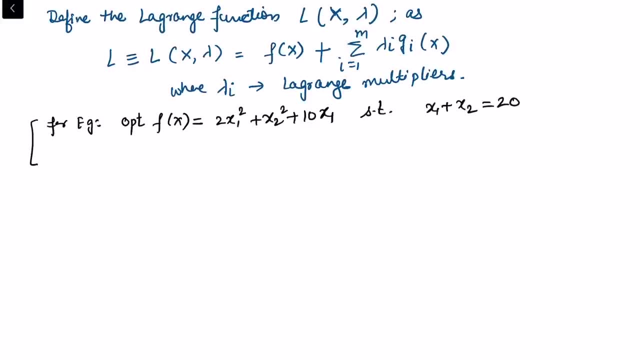 constraint x1 plus x2 equal to 20, and then we can take, let's say, one more constraint, 2x1 minus x2 equal to 6, and then we have x1, x2 greater than equal to 0. now for this non-linear programming. 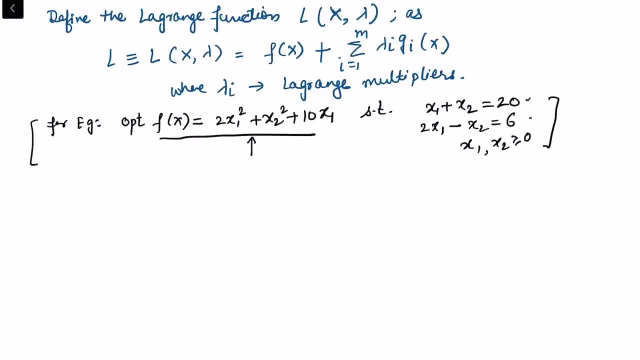 problem. as you can see, the objective function is non-linear. here the constraint are linear. so the first constraint: here i will write it as g1- x, which is x1 plus x2 minus 20, equal to 0. and the second constraint: here i've considered it as 2x1 minus x2 minus 6, equal to 0. now these: 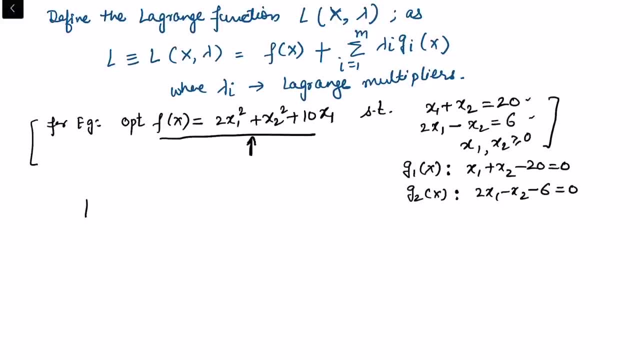 are the two constraint and this is the objective function. so for this lagrange function will look f of x. so here we'll first put f of x plus 10 times x1 plus. now we see that lambda i multiplied by the constraint. so for each constraint we will have a multiplier, so i: 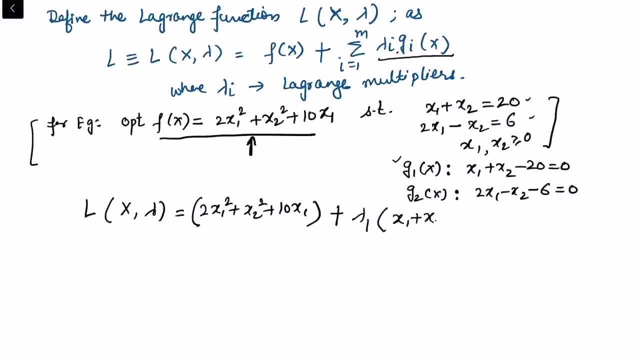 will take lambda 1 into the first constraint, x1 plus x2 minus 20, and then i will add plus lambda 2 into the second constraint, 2x1 minus x2 minus 6, so we can add as many as multiplier, depending upon how many. 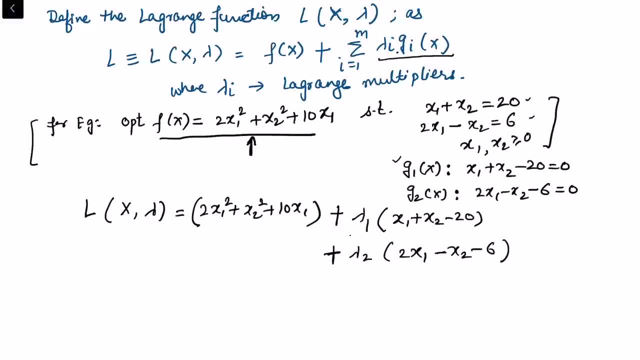 constraint do we have? if there is only one constraint, then there will be obviously one multiplier. so this is how we will carry on. so in general, this will be the notation we will use. if there are m number of constraint, then we will add a lambda i multiplier. so there are m number. 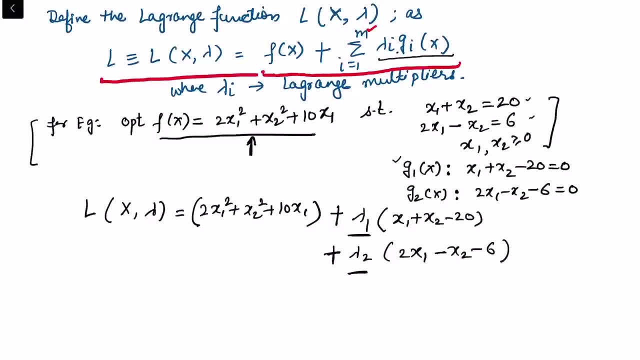 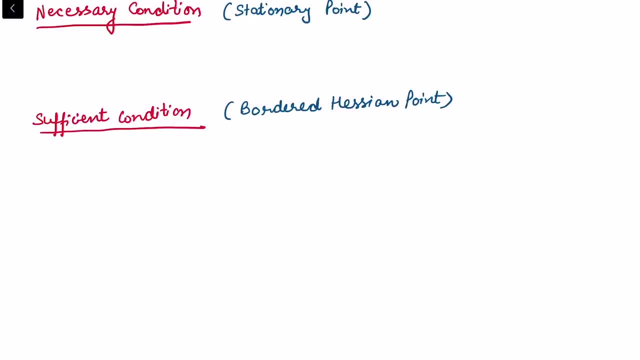 of multipliers that we have added now. this is the single objective now and we want to optimize this, so this is to be optimized. so before we jump to the question, we'll look at what are the necessary condition, what are the sufficient conditions. so, for the necessary condition, we, as we see that now, 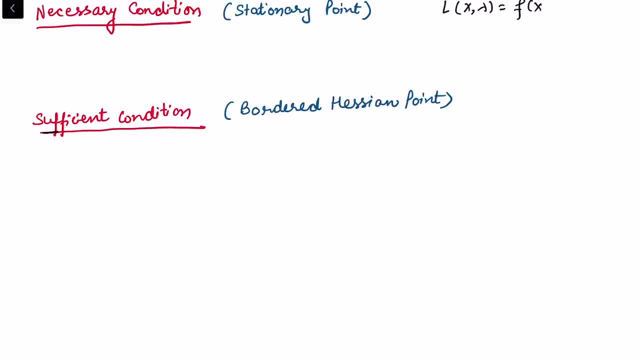 our lagrange function. this consists of f of x plus lambda i times g i x. okay, and then we can i varying from 1 to m. so here we will consider again the partial order derivative, as we did in the earlier cases: lambda l with respect to lambda. 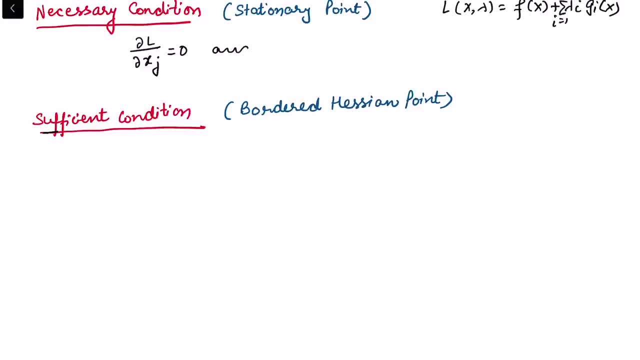 x, j equal to 0 and we will so here. j varying from 1 to n. so, considering that there are n number of decision variables and curly l with respect to curly lambda, i equal to 0, so we consider i varying from 1 to m. there are m number of constraints, so find the solution from there and this will allow. 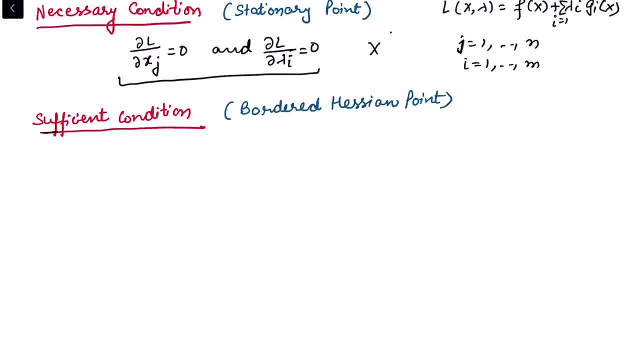 us to find the stationary point. so we will first find a stationary point, capital x, and correspondingly we will also find the lambda star. so, solving these equation, we will find these points and this we call as stationary point. now stationary point can be a point of maxima or minima. so for that we will look at the sufficient condition and we also 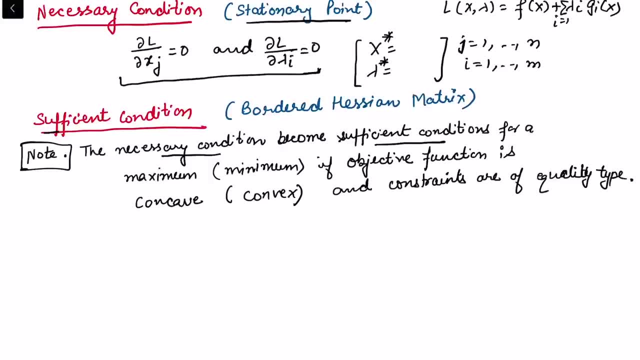 note that the necessary condition becomes a sufficient condition. so if the objective function and the constraint which we have considered for the equality type, if they both are convex, then we will say that the function will attain a relative minima, and if the objective function constraint are concave, then the function, the objective function, will attain a maxima. i will 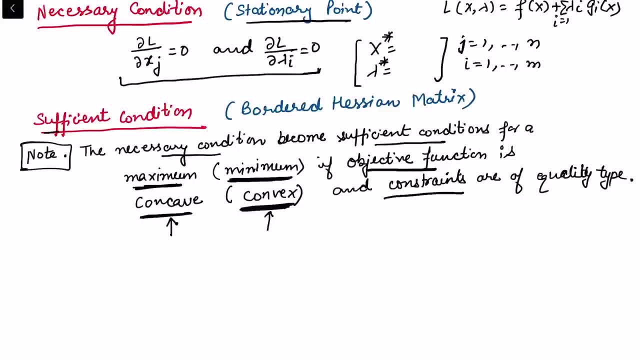 talk about the convex and concave in my next video, but in this current video we will classify the sufficient condition. i have not included the proof, but we will be using the bordered hessian matrix. so, as we did in my last video class, there was a matrix associated with the quadratic form and 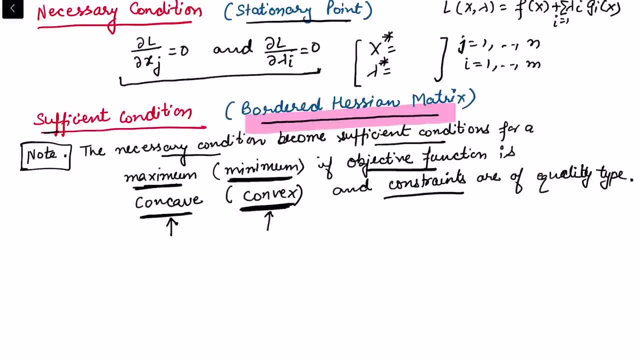 non-quadratic form. so we will talk about the convex and concave in my next video, but in this current video class there was a matrix associated with the quadratic form and non-quadratic form. similarly, now we will look at the classification of this bordered hessian matrix and we already have a 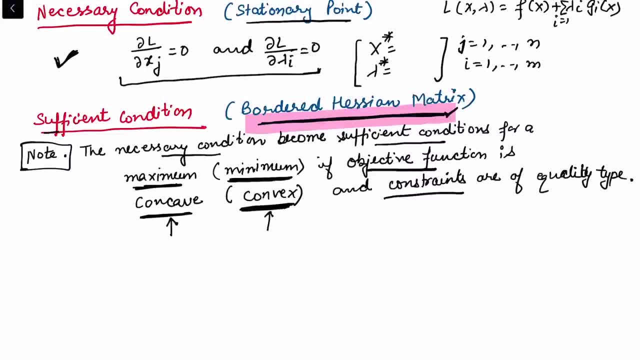 stationary point now, based on the classification and based on the result, we will conclude with whether this have a maxima or minima. so let me to first define what is hessian matrix, then we will write the result and we will follow up this by an example. so we defined hessian bordered matrix and 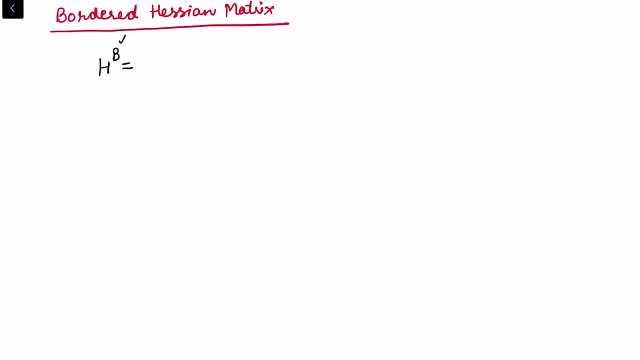 we use the notation hb. this b just stands for the bordered hessian matrix. and again, hessian matrix is a partial order derivative. so let me to first write its closed form. it is 0, p, p transpose and q. so this will be a matrix of order m plus n, cross, m plus n. so this would be the order now: 0 here. 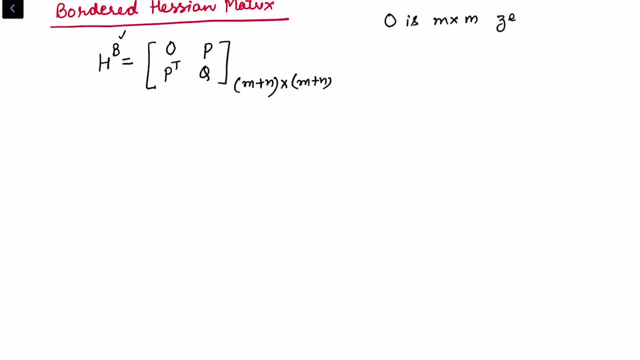 is a m cross m 0 matrix. so this is here. it is just a notation of 0, but this will be actually a 0 matrix. capital p: this is again a matrix of the partial order derivative which is due to the. so we know that fx, this is the objective function, and gix, these are the constraint. 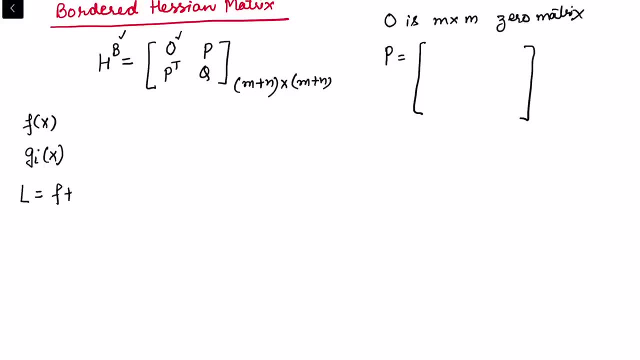 and l is the lagrange function, which is f plus lambda 1, g1, x plus, so on up till lambda m, g, m, x. so this is how we have constructed the lagrange function. now for the p matrix. we only require the first order, partial derivative with respect to all variable of the constraint. 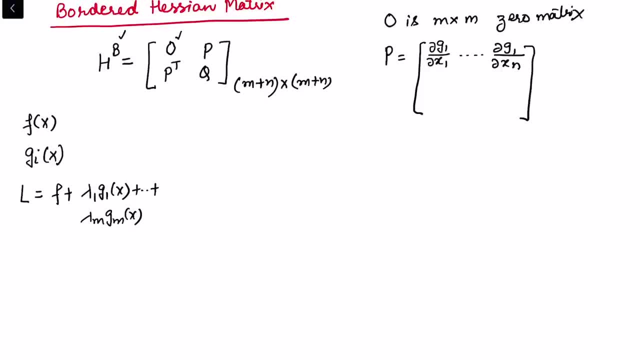 so let me do: first take the first constraint and then take the partial order derivative with respect to all decision variable. then we take g2, second constraint, and take the partial order derivative with respect to all decision variable xi. and finally we continue and take the partial derivative of the mth constraint with respect to all decision variable. so this is the p matrix. so 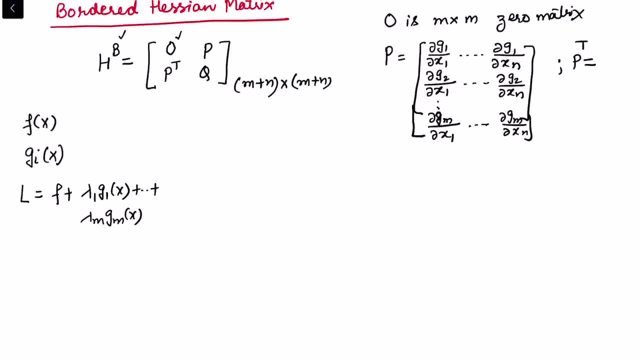 and then we will obviously can write p transpose. once we know what is speaking of matrix, we can write p transpose. q is the- again second order- partial derivative. but now this is with respect to the lagrangian function. so in the lagrangian function we have the partial, again the 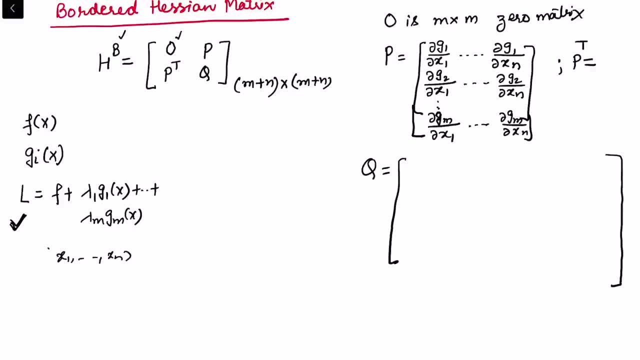 decision. variables are from x1 to xn, so we will construct first the lagrangian partial order derivative with respect to x1 and then take first row with respect to x1. okay, so let me to write one by one so that there is no confusion. first write the partial order derivative with respect. 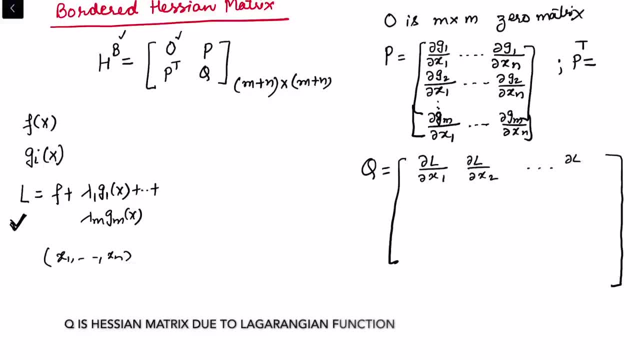 to all decision variable curly l with respect to curly xn, and repeat this process for n nth one. so we will repeat n times. so there are n number of rows and n number of columns. so this is first order, partial order, derivative. these are same terms. the only difference is here i am writing. 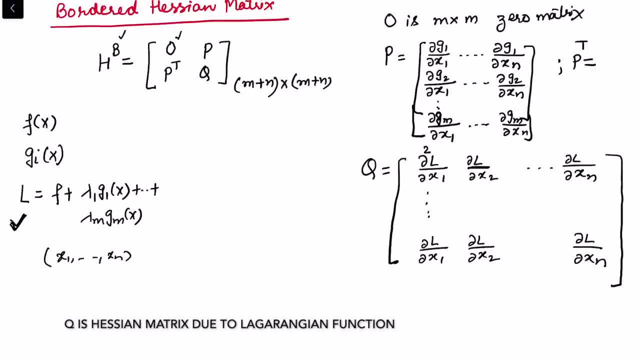 now i want to take basically first row Care attempt to�undi. So when i again first row with respect to x1, this will become the square. here i will take with respect to x1 and here also i will take with respect to x1. in the second row i will consider. 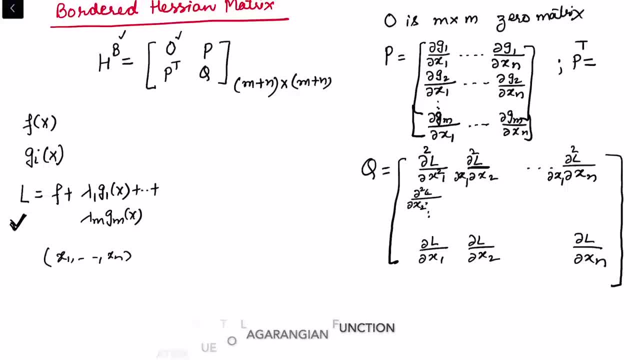 the partial order derivative with respect to x2. so this is x2x1 and this will be curly square l with respect to curly x2 square and this will be curly square l upon curly x2 with respect to xn. okay, continue a third row with welcoming the other. 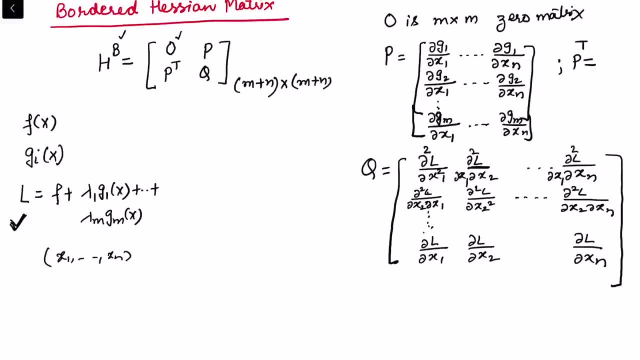 row with respect to x3 and the last row with respect to xn. so these are the partial order derivative mixed partial order derivative we are supposed to get. this is exactly similar to haitian matrix. now this is what we call it as bordered haitian matrix. so now we follow this. 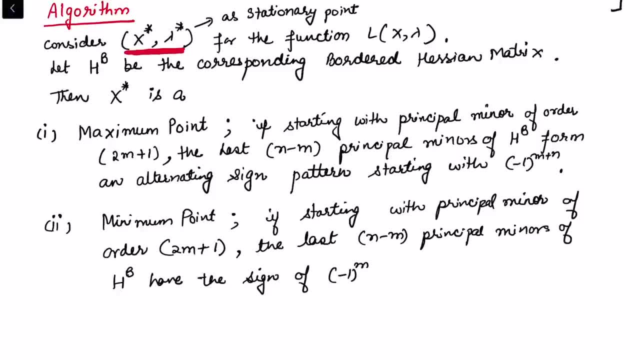 algorithm that we have found the stationary point- and here i'm just writing, considering x star and lambda star as a stationary point, which we have found by putting the partial order derivative with respect to all decision variable xi equal to 0, curly l with respect to curly xi, j equal to 0. 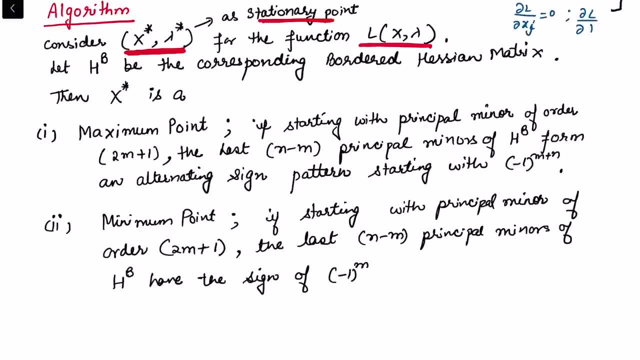 j varying from 1 to n and curly l with respect to curly lambda i, equal to 0. solving these equation, we will find x star and lambda star and let h star hb be the corresponding bordered haitian matrix, and we will classify this bordered haitian matrix as giving us the point x star as a point. 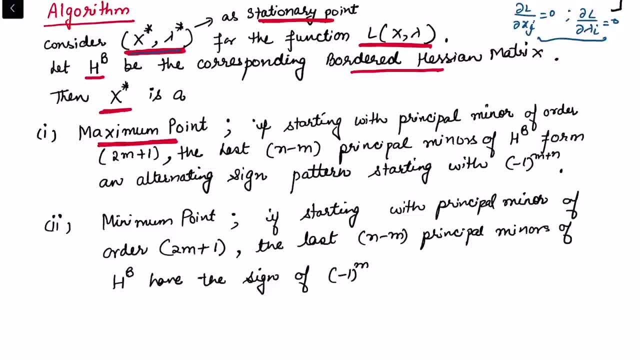 of maxima or minima. so this you is a point of maxima, or we'll say maximum point. if, looking at the haitian bordered matrix and we start at the principal minor of order 2m plus 1, so we know the principal order minor is 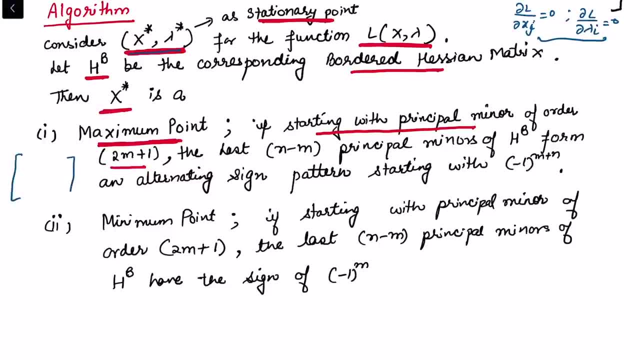 say, for example, we consider a matrix of this type- it has to be a square matrix- then we start considering the first element and then we take the determinant of the 2 cross 2 matrix, then we take the determinant of 3 cross 3 matrix. these are called the principal minor order. 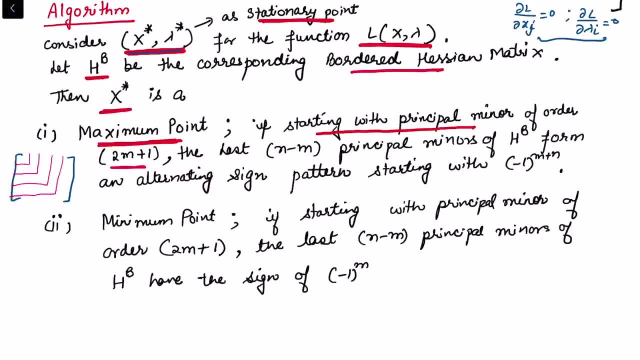 so we have to consider the principal minor of ordered 2m plus 1. so if there are one constraint we will start looking at the third matrix. so if there is, m stand for the number of constraint. so 2m plus 1 will become third constraint. so look at the 3 cross 3 ordered. 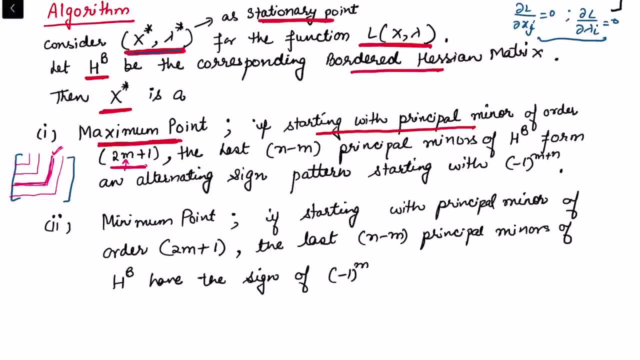 this principal minor determinant and to the last. so then, calculate 4 cross 4, calculate 5 cross 5, depending upon how many further ah minors are coming in that particular matrix matrix. so to the last, n minus, m principal minus, and if they form an alternating sign pattern, so 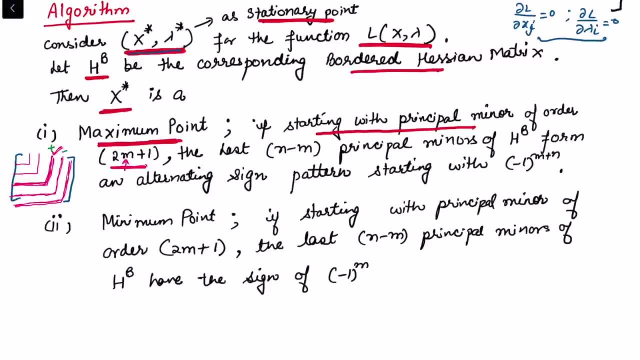 for example, this have the plus sign and this have a negative sign and this have a plus sign. so they form the alternating. but the starting sign should be minus 1 to the power, m plus 1. so it depends whether we can have a starting sign like plus, minus, negative or we may have. 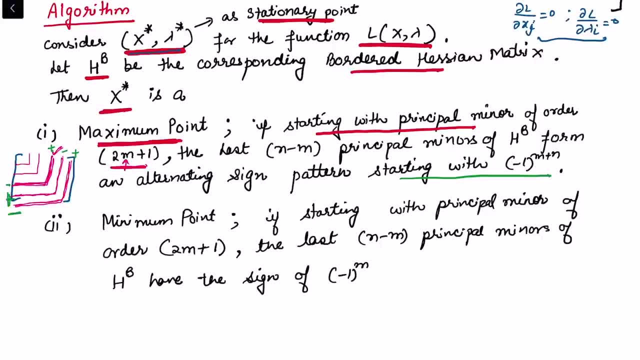 minus plus, and then we can take a negative sign. so the starting sign will depend upon this symbol, which is minus 1 to the power, m plus n. similarly, it will have a point of minima if, starting with the principal minor of order, 2m plus 1 to the last n, minus m principal, minus the hessian border. 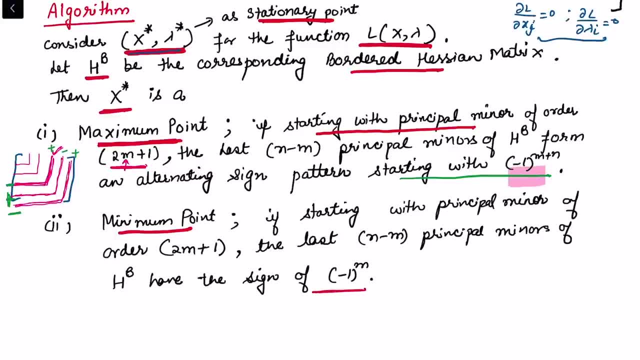 matrix have a sign minus 1 to the power m. so either these sign are all positive. so in this either all positive or they may be all negative. again, it depends upon the number of constraint. so if the number of constraint are odd, so if there are one and three constraint, we will always get a negative sign. 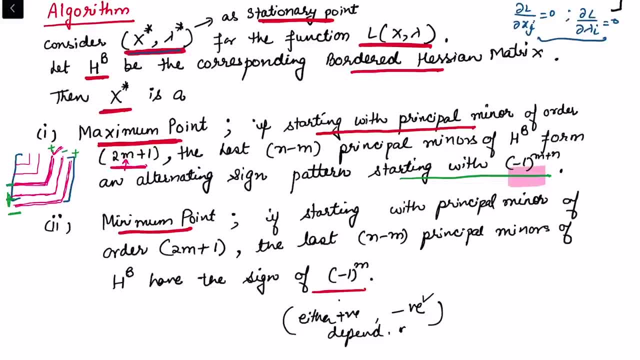 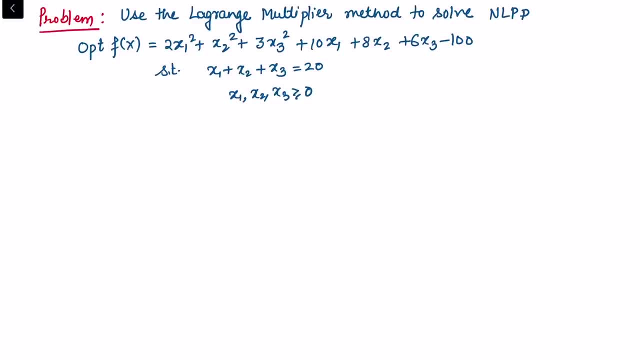 or it. if there are number of constraint are even, then we will always get a plus sign. so now let's take an example and implement this. so consider this problem. here i want to use lagrange multiplier method to solve the non-linear programming problem and we have an objective. 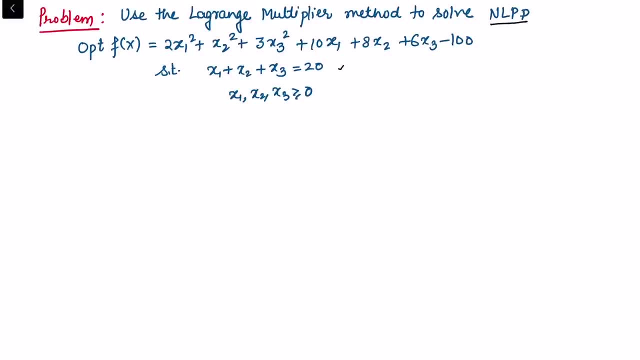 function and we have an equality constraint. so for this problem, let me to first construct the lagrangian function, and for this we will construct a lagrange function: l capital, x lambda. so this is f of x plus. there is only one constraint, so i will only consider: 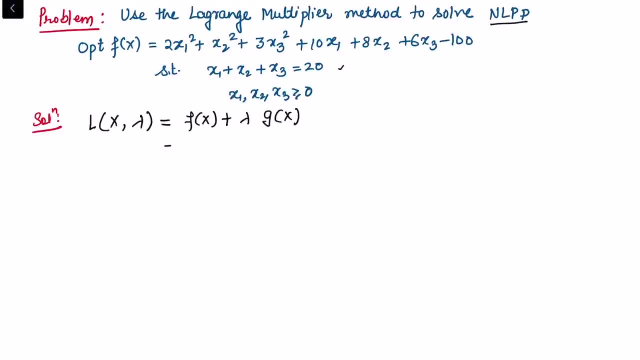 lambda times the constraint, that is g, x. so we can consider now: f x is 2 x 1 square plus x 2 square plus 3 x 3 square plus 10 times x 1 plus 8 times x 2 plus 6 times x 3 plus x 4 plus x 1 is 2 and x 2 because sm. felwtime constraint with a function of f x is therefore we will construct l capital x, so i will no constraint and we will construct a lagrang function only. so i will consider lambda constraint for g x. so we can consider now: f x is 2 x 1 square plus x2 square plus x 3 square plus x 3 square plus 10 times x 1 plus. Спасибо. 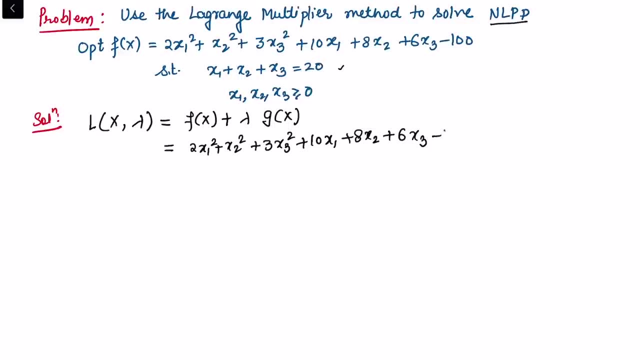 you for understanding Within this question, what kind of constraint you are present here. so today we are going to look for examples x2 plus 6 times x3 minus 100. so this is f of x. that's the value for f of x plus we want. 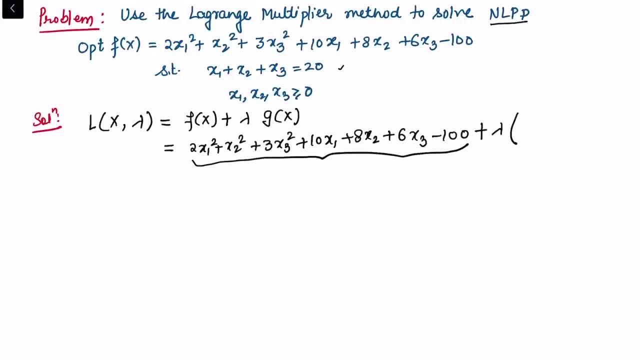 to take lambda time g of x, and, as i have said, constraint are always considered with the equal to zero sign. so constraint here in this case is x1 plus x2 plus x3 minus 20. so now we find the necessary condition for the stationary point, and for this i require curly l with 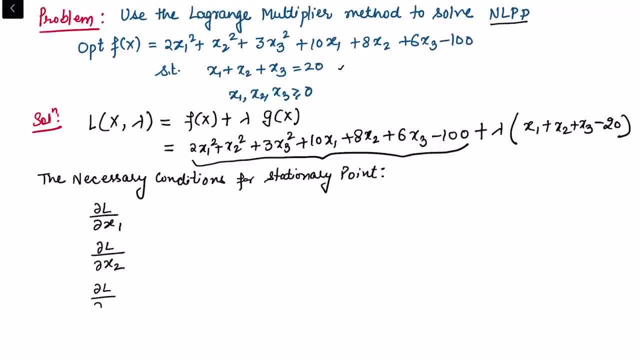 respect to curly x1, x2, and then i also require curly l with respect to curly x3. there are three decision variable and we also require curly l with respect to curly lambda equal to 0, so put all these equal to 0 once we write them. let's first find curly l with respect. 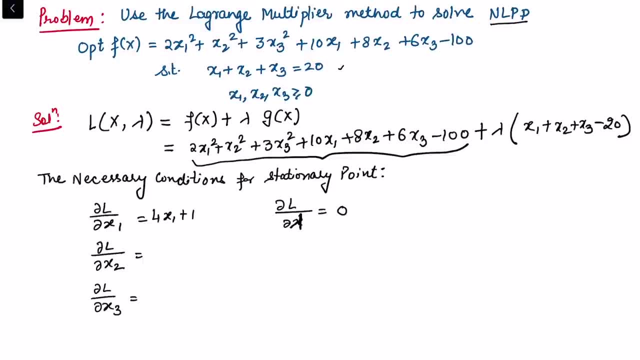 to curly x1, so this is 4x1 plus 10, and then one is coming from here, so we will have plus lambda equal to 0, and then, similarly, i will find: okay, let me to first find, with respect to x1, kali is not a variable for all. right, we will find it. similarly, i will find the 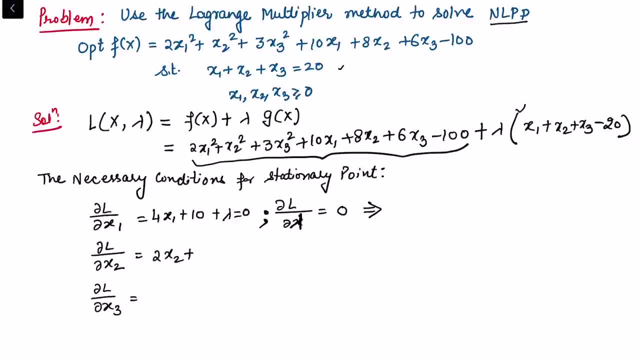 x2, so this will become 2x2 plus 8 plus lambda, equal to 0. and then we have with respect to x3, so this will become 6x3 plus 6 plus lambda, equal to 0. and with respect to curly l, with respect to: 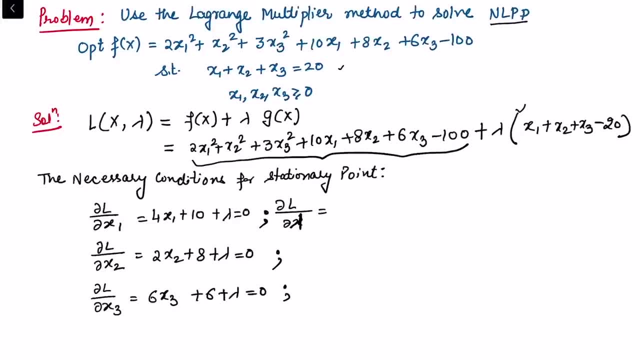 curly lambda. let's first find this also. so with respect to lambda, we can see this whole will come. so this is x1 plus x2 plus x3 minus 20 equal to 0. now we solve these equations. so we will write: solve these together, or we can say: solve these simultaneously, so solving these simultaneously. 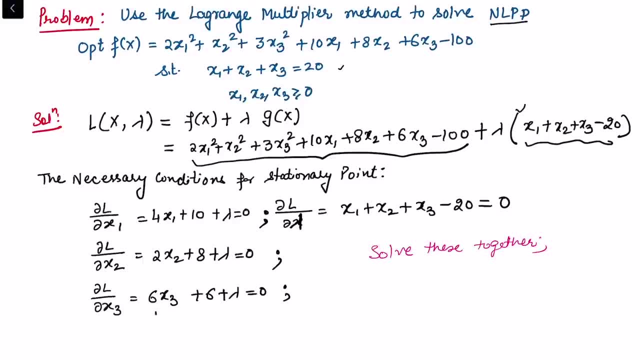 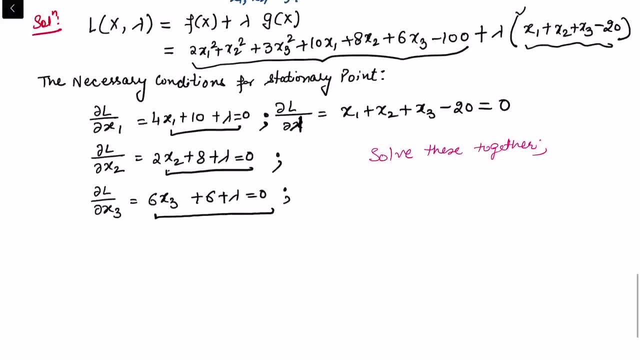 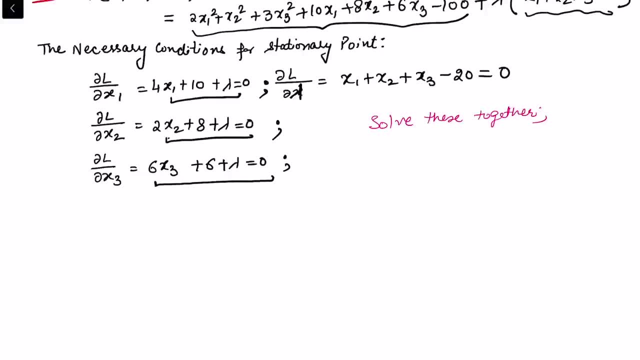 and subtract among each other to reduce these equation. so let me to write these as 1, 2, 3 and this one as 4. so from 1 we can calculate that x1. this is minus of 10 plus lambda by 4. 1 and then 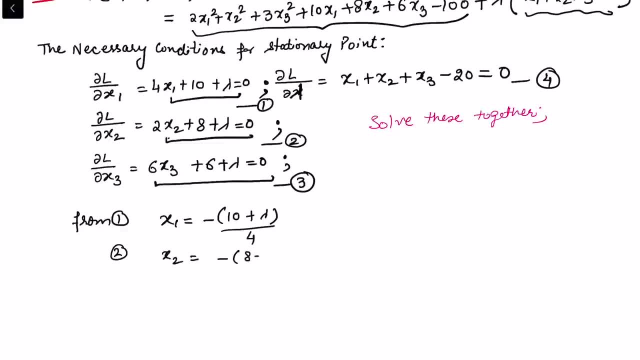 from 2 we calculate x2, which is minus of 8 plus lambda by 2, and then from 3 i calculate x3, which is minus 6 plus lambda by 6, and put these in 4, put these in 4, so when you put this into 4, so you see that this is x1. 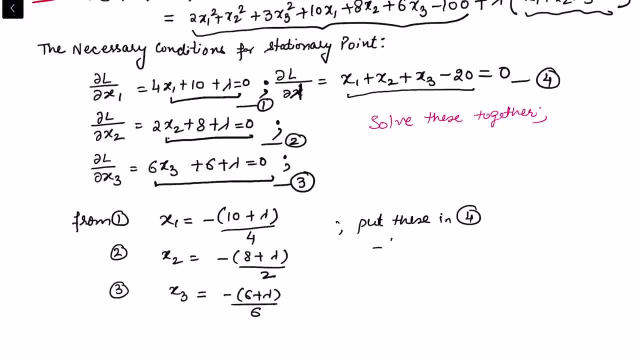 plus x2, plus x3 minus 20, so x1 value is minus 10 plus lambda by 4, and then you have x2, which is minus of 8 plus lambda by 2, and then we have minus of 6 plus lambda by 6. that's value for x3. 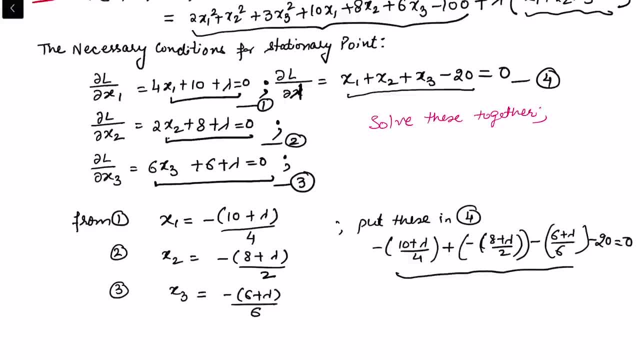 minus 20 equal to 0. so in this there is only a minus of 8 plus lambda by 2, and then we have only one variable and we can solve for lambda. so we solve for lambda and we get: lambda is equal to minus 30. now, once we got the lambda, we can find x1, x2, x3. so the first thing is that we need to 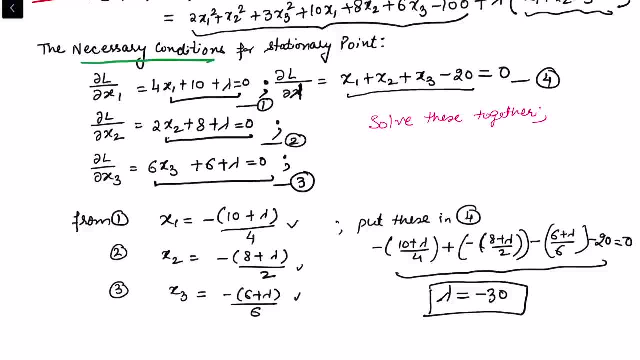 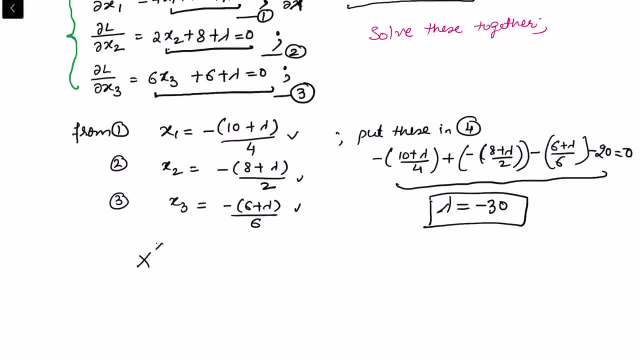 look at the question and we need to know how to solve these equations. so there, we need to apply little algebra, our usual maths. so now, once we found these x1, x2, we can find the stationary point, and the stationary point is 5, 11 and 4. so and we know the. 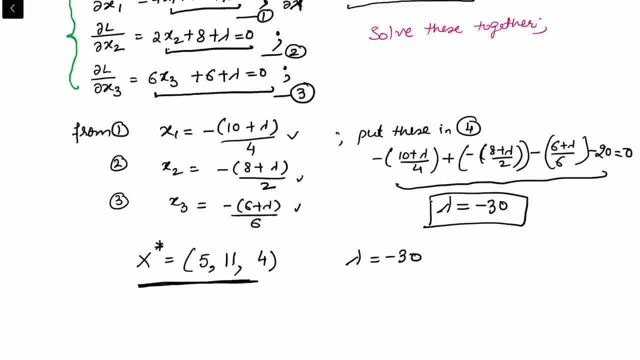 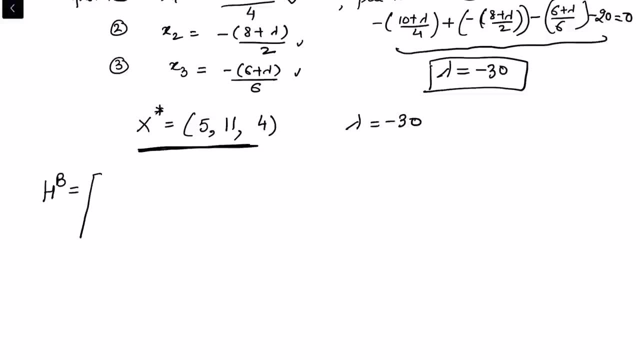 lambda is minus 30. so basically, we are looking for this x star. now we got the stationary point and now we are looking for the haitian bordered matrix. for the haitian bordered matrix, we have this as 0, and then we got p, then we got p transpose and then we have q. so this was the. 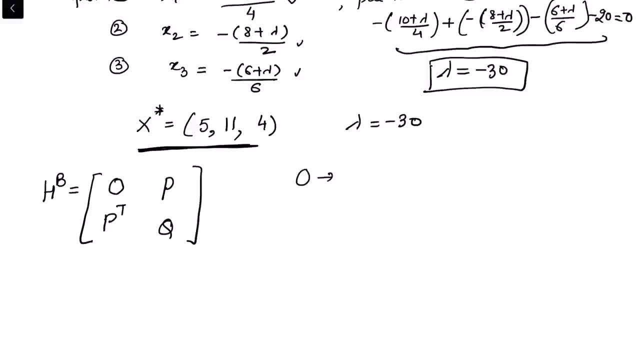 haitian bordered matrix and 0. this was the m cross m 0 matrix. so in this case, m cross m. this was the number of constraints. so this m stands for number of constraint. now there are, there is only one constraint, so so we will only have a 0 entry here. okay, so maybe we can just write it like this: 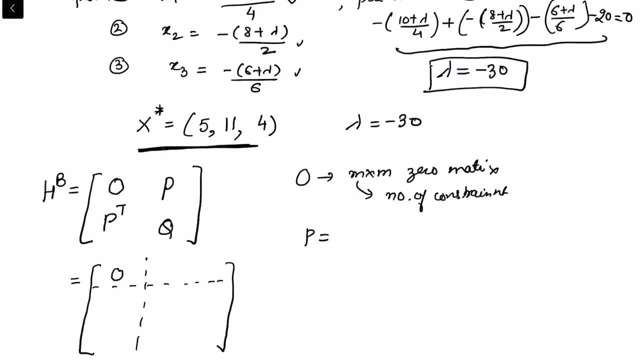 one for p. this is the gradient of the constraint. so now there is only one constraint, so we will only have a one row. so first constraint with respect to x1, and then we have first constraint with respect to x2, and so on. we'll have the first constraint with respect to xn. so we have now. 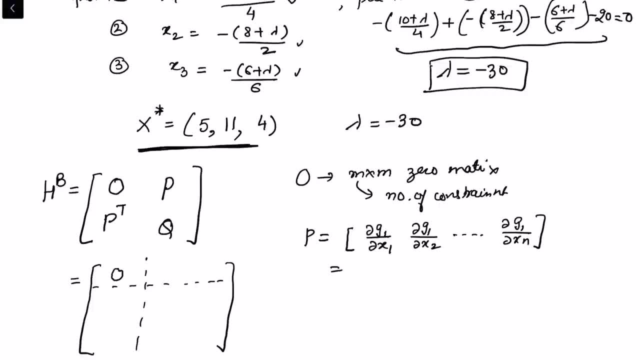 there are only three decision variables. so basically this will remain up till curly g1 with respect to curly x3. so we'll find out the partial order derivative with respect to x3. the constraint that we have here is: we will write the constraint here. constraint was x1 plus x2 plus x3 minus 20, this was the constraint. so if i found the partial, 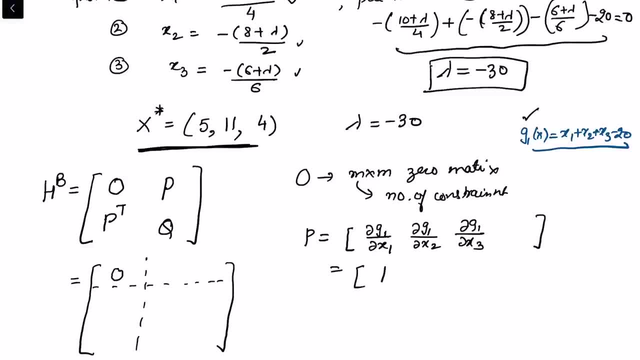 order derivative of this constraint: with respect to x1, i will get 1. with respect to x2, i will get 1. with respect to x3, i will get 1. so this is 1, 1, 1. so now these entries will go here: 1, 1, 1 and then the row, so this p matrix, which is now a row. 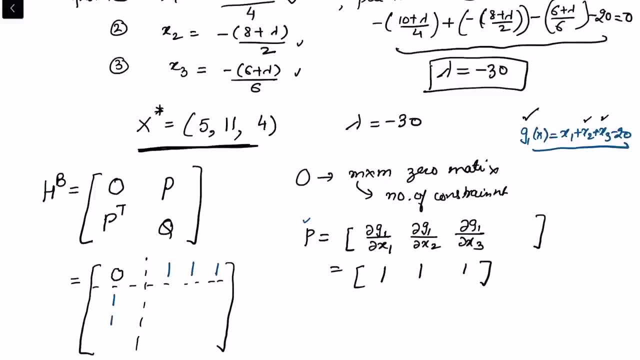 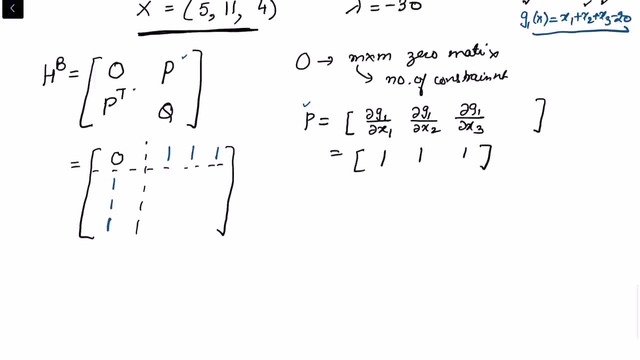 its column, its transpose will go here. so this is p transpose, so this is p, and then we got p transpose. now i need to find what is q for q. i require now the partial order derivative of the lagrange function. so let me to again look back. what was the lagrange function? l is this and we 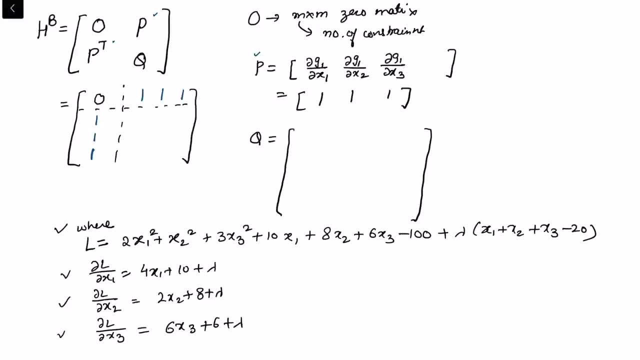 can see here. firstly, we have fastly l minus 80, and then we will write the partial order derivative of con she and then we will write: Итак, this is she, and then we will get back The partial order derivative and the function fewer than or equal to minus. 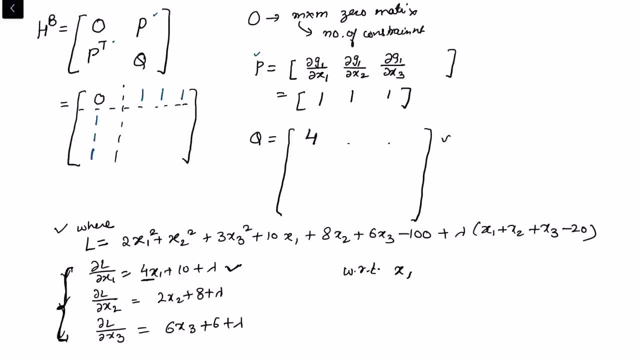 0 minus feet two, and we basically, alsofastly, we will divide it into elements which are 3 cube and 2 square root. 2, 1 and minus 4 is equal to minus x22 minus 2 vertical integral, or which means squaredude Serve times w, times square root xn and picin t times square root. 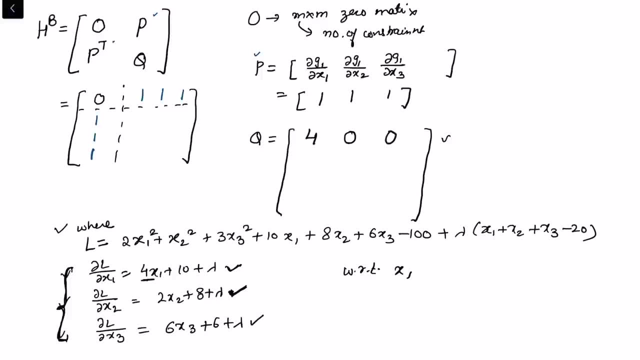 term. so this is 0. here also there is no partial order derivative with respect to x1 we can find. now repeat the process. we again want to find these partial order derivative with respect to x2 and then put it in the second row. so this is 0, 2 and then we got 0. then in the third row, find. 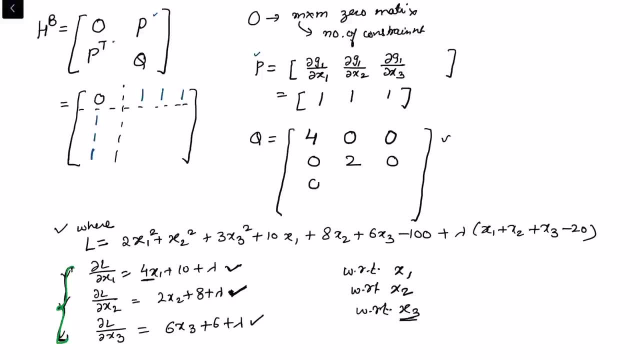 the partial order derivative with respect to x3, so this will go here: 0 0 6. so we got q and put the q here. so this is 4 0 0 0. 2 0 0 0 6. this is the bordered hessian matrix and we will now. 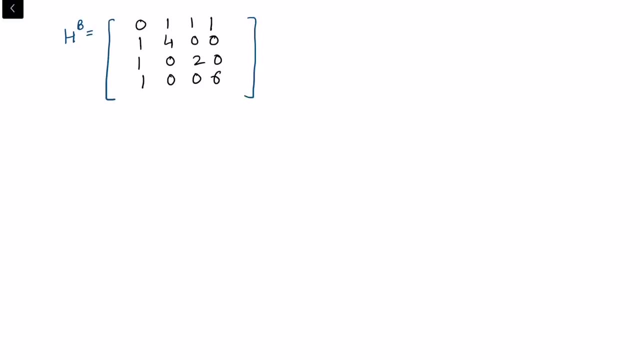 check the hessian border matrix: principal minor. so here we again see n- this is the number of variable in the problem- and m. so the variables that we have used is x1, x2, x3 and m. this is the number of constraints. so we want to start by checking the principal minor determinant. 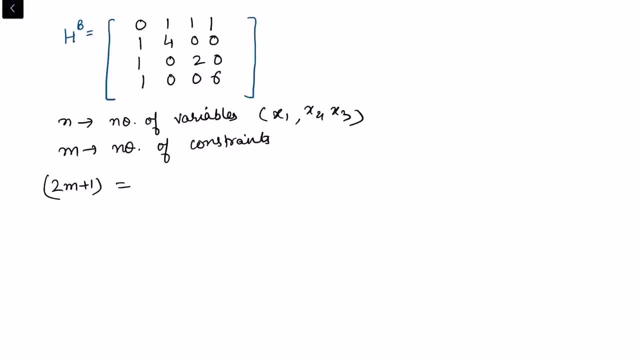 4 from the order 2m plus 1, and here m value is 1 and n value is 3, so 2 into 1 plus 1. so we want to start from the 3 cross 3 order determinant. so we will check this one 3 cross 3 order and let me to. 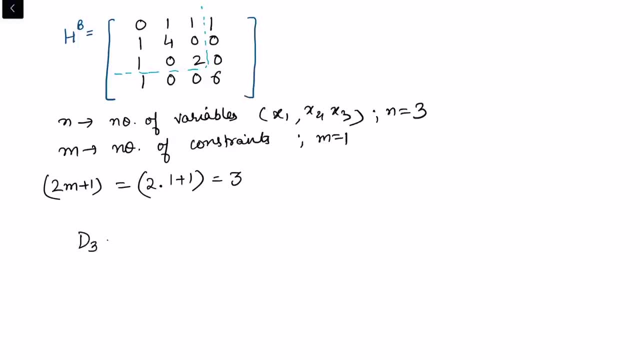 just write this as d3. so d3, which is the determinant of 0, 1, 1, 1, 4, 0, 1, 0, 2, and if i find this determinant, this comes out to be minus 6, and then we continue till the last. so last would be finding the principal minor determinant of. 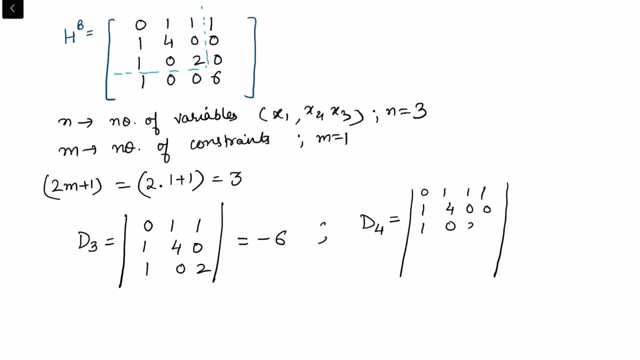 4 cross 4. so this is 1 4 0 0. 1 0 2 0. 1 0 0 6. if i find the determinant of this, this will come out to be minus 44. now we notice that both these signs are negative, so they does not form an. 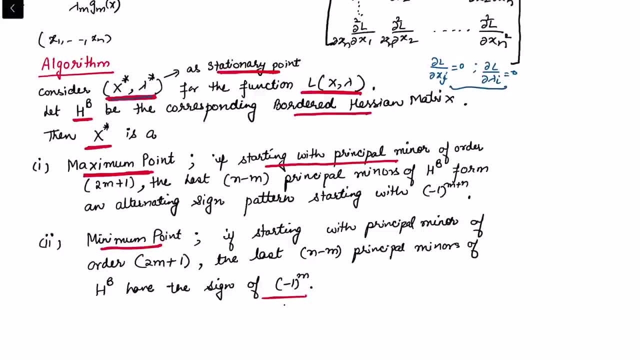 alternate sequence. so if we look at this criteria again, the first one to have a maximum point, we need to have an alternating sequence. so this one is cross 4 and this one is negative, so this one is crossed off. we may look at the second one if the hessian border matrix form the size minus 1 to the 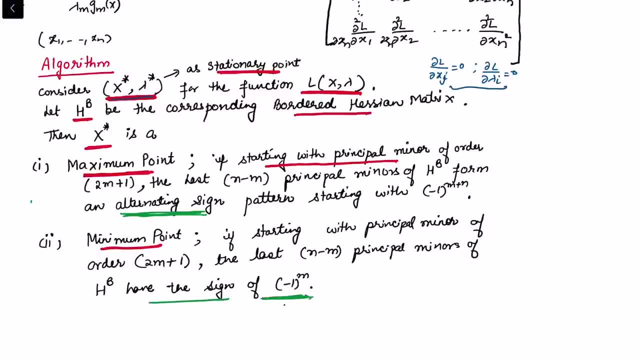 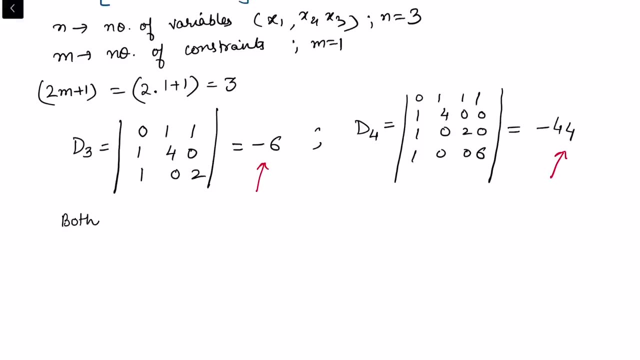 power m. all the sign are to be minus 1 to the power m. then we say that it has a point of minima. so in this case we have one constraint and the sign is minus. so it fits into this category that the stationary point is a point of minima. so we can write both d3 and d4 have sign of minus 1 to the power m. 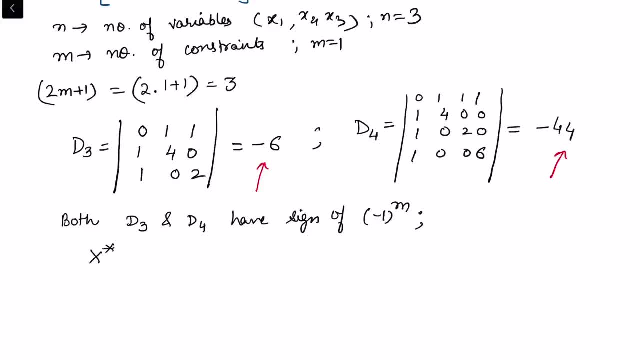 so we conclude that x star. this is a point of minima, and to find the minimum value now, we can just simply substitute this in the objective function, because objective function was that what we wanted to find and objective function was given by f of x. so we'll calculate f of x star. 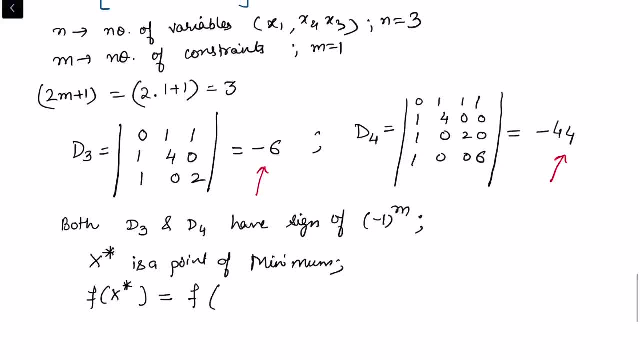 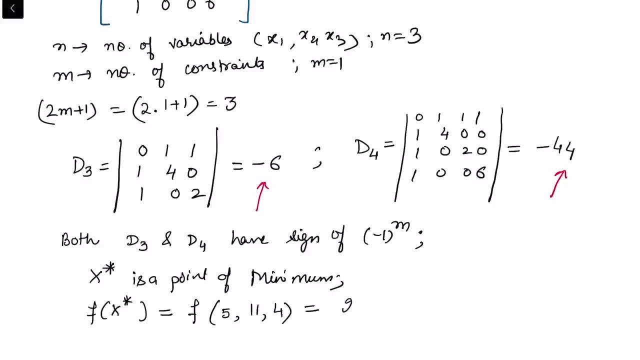 and by substituting f, the x star point that we have calculated. this was 5, 11 and 4, so substituting this, we will get that this function value is 281. so this is the stationary point, is a point of minima and this becomes our optimal value. so this is how we can find the optimal solution. 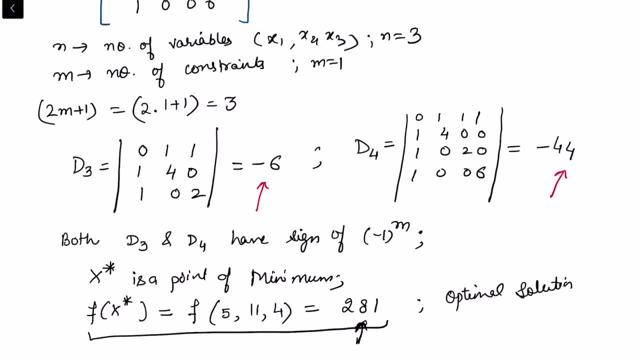 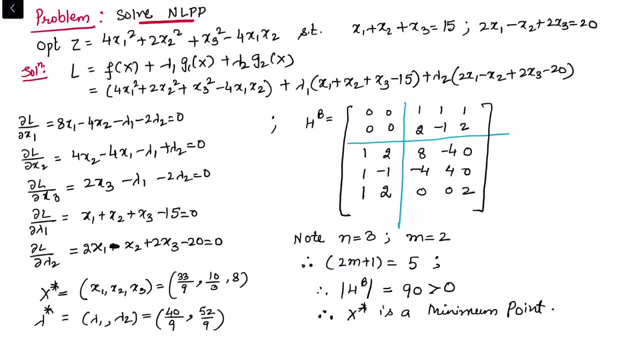 for the non-linear programming problem with the equality constraint. and before i end let me to take one more example. so in this problem we again consider one more non-linear programming problem. we got objective function and there are two constraints. so we first construct the lagrangian. 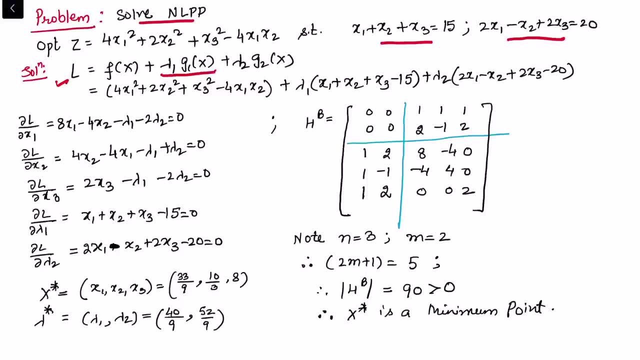 function l, which is f of x plus lambda 1 times g 1, x plus lambda 2 times g 2 x. now to find the stationary point. these are the necessary condition. so take the partial order derivative with respect to x 1 x 2, x 3. lambda 1, lambda 2. 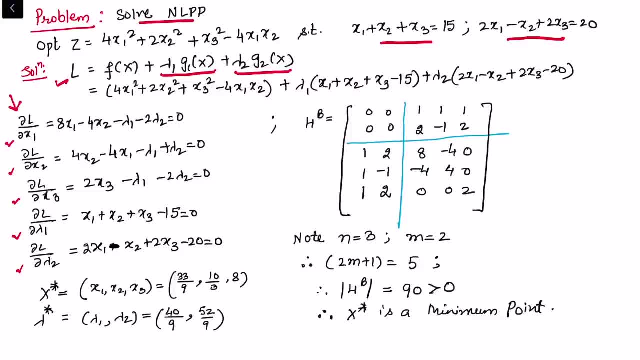 and we solve these simultaneous equations, solve these equations and we find x star and we find lambda stars. now this is the stationary point, and for this stationary point it can be a point of minima or maxima. so for this we identify it into haitian border matrix. 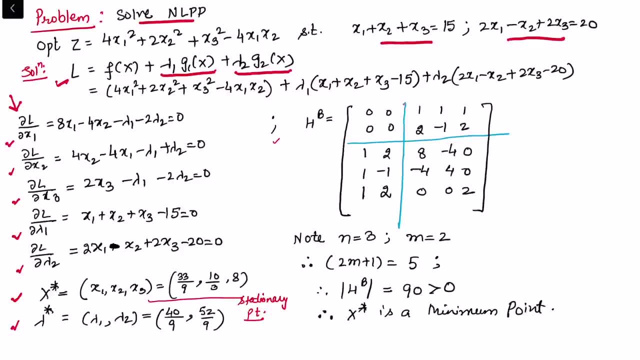 we look at the block so we can see that this is a two cross two block because there were two constraints. so this is a zero matrix of order two cross two. then this one is a p matrix and its transpose goes here in this column. so one, one, one, two minus one. we can see from: 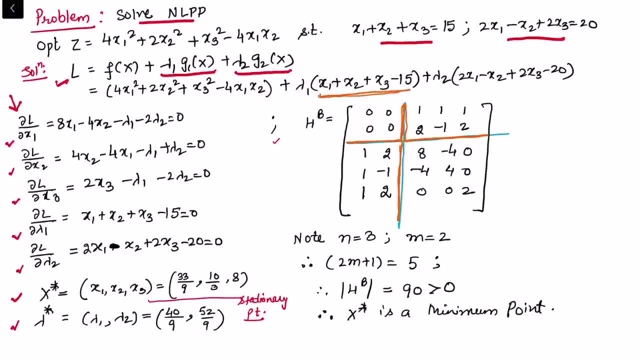 the constraint: uh, this will go partial order derivative with respect to x 1, x, 2, x, 3, so this is one one one here, and then in the second constraint we again repeat the partial order derivative with respect to x1, x2, and we will put it on the second row here. so this is how we got. 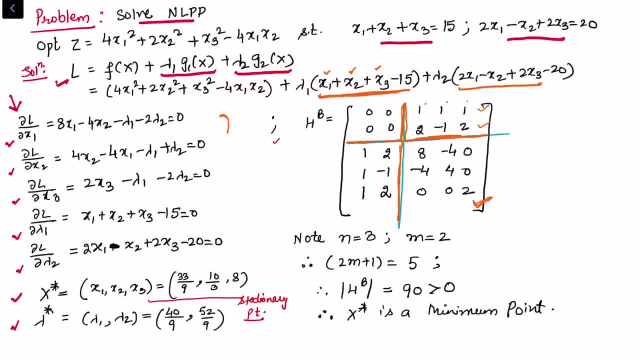 this one is the lagrange function that we have already calculated. their partial order derivative: first row with respect to x1, so 8 will come here, then minus 4 will come here, and in the third row there is no x1. so here there is no x1. so this is why 8 minus 4, 0. similarly, then we find the: 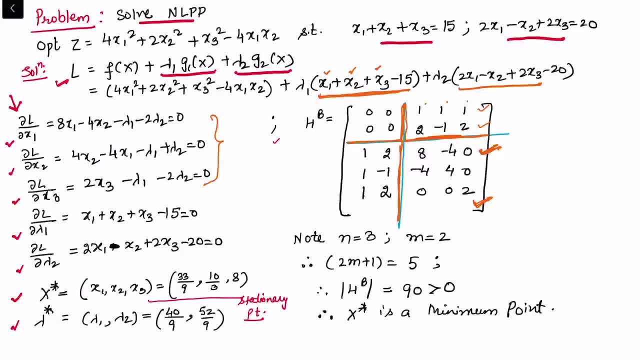 partial order derivative of these, again with respect to x2. so for x2 this is minus 4 x2, you will have 4 here. there is no x2 in the third, third equation, so we will put a 0 here. then we will repeat again partial order derivative of these equation with respect to x3 in the first there. 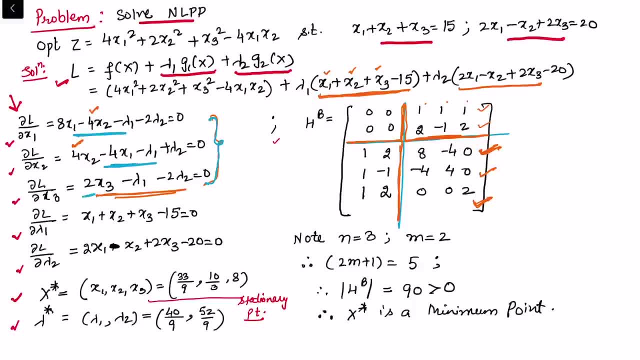 is no x3, in the second there is no x3, and in the third we got 2, so that is why it is 0 0 2. we have now, then, written the hessian border matrix, and we will now classify its determinant. so for the determinant we need, 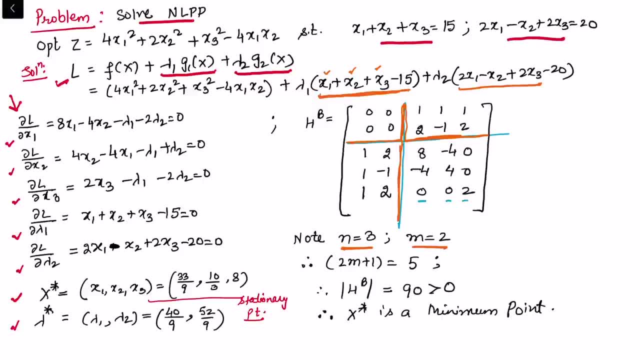 to look what is n, n is 3, m is 2, so we need to start looking the principal minor determinant of this order till the end. so when i put m is equal to 2, we got 5. so which means that we need to take a 5 cross 5 determinant at the starting, but the maximum order is only 5. this means we 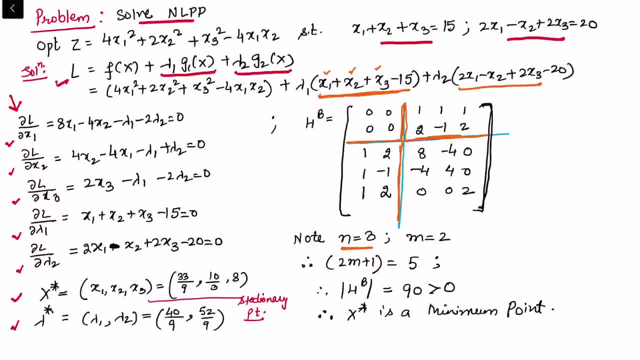 need to only calculate the 5 cross 5. that means hessian bordered determinant. so we calculate this determinant, which is 90. this is positive and it it is positive and it also fits into the sign of minus 1 to the power m. so this is minus 1 square and the sign is positive. so that is why we conclude. 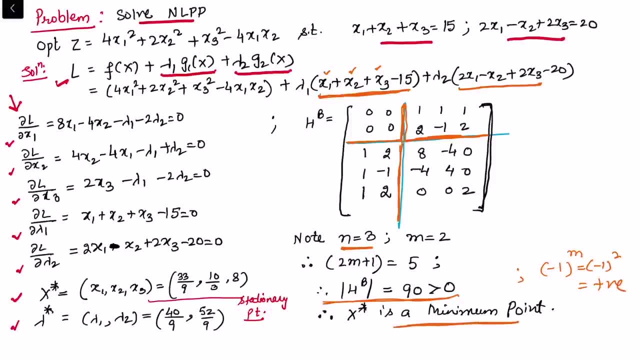 that this is a point of minima. we could have checked this for the other case. also for the maxima, it should follow the sign minus 1 to the power, m plus n. but m plus n will give me 5, and so this sign should be negative. so, although alternating,